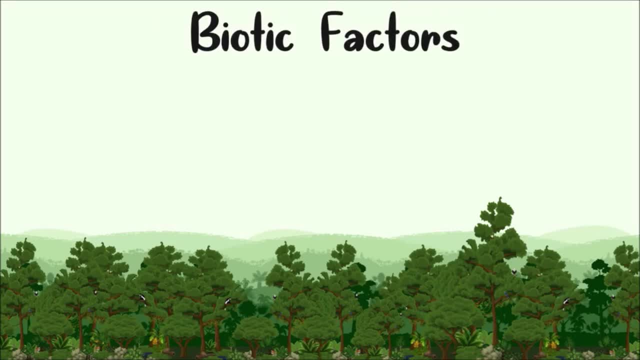 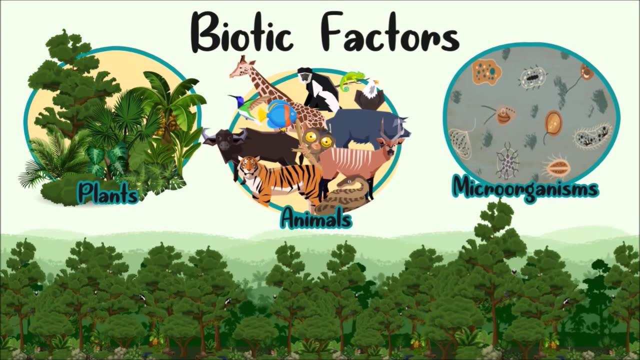 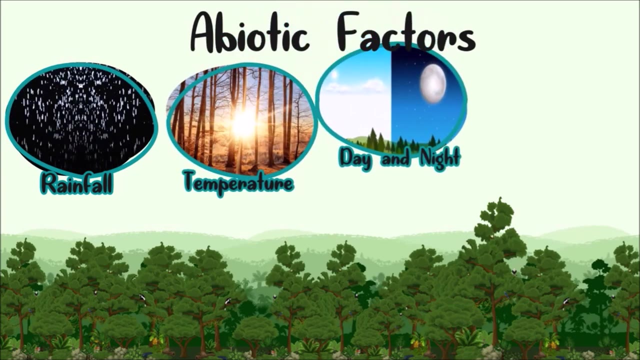 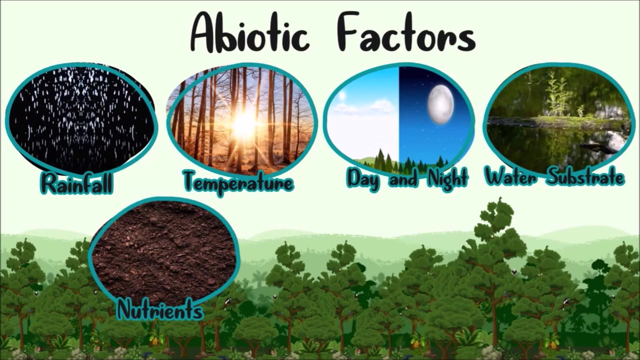 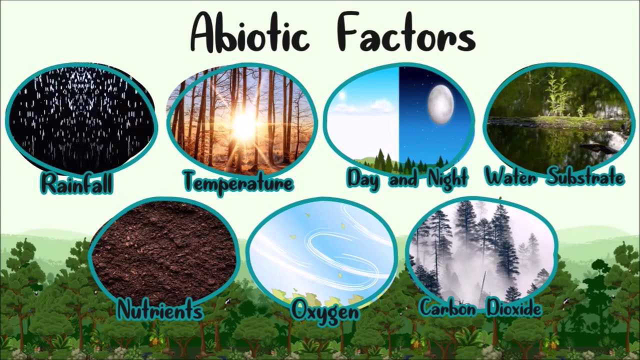 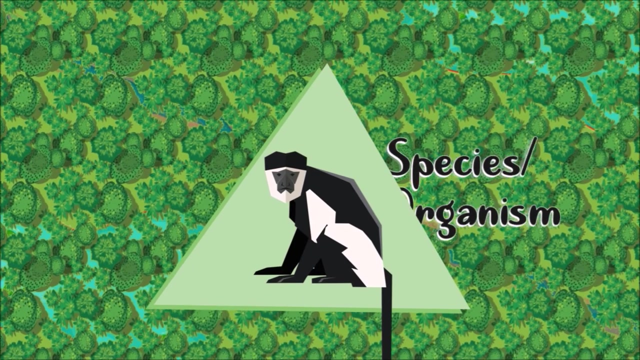 biotic factors may be plants, animals or other organisms. well, some examples of abiotic factors are rainfall, temperature, length of the day and night, water, substrate, nutrients, oxygen, carbon dioxide and many more. the living part of an ecosystem consists of different species or organisms. each species is a part of the 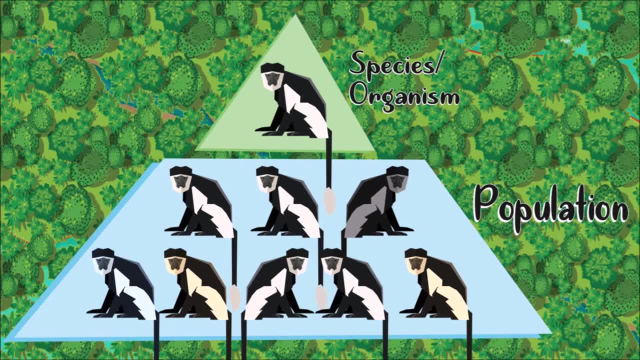 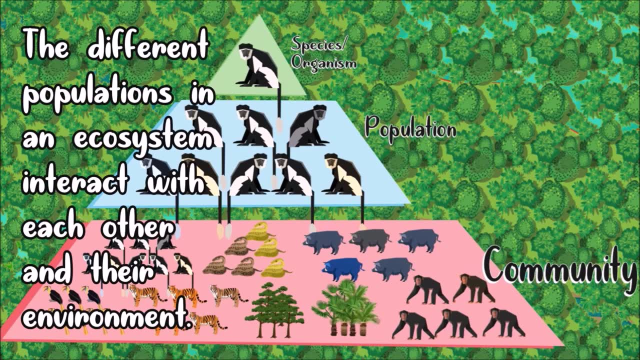 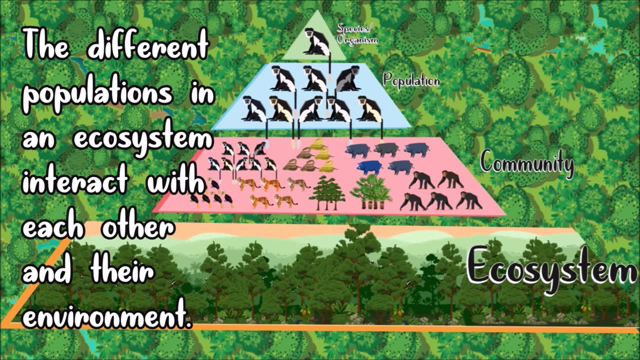 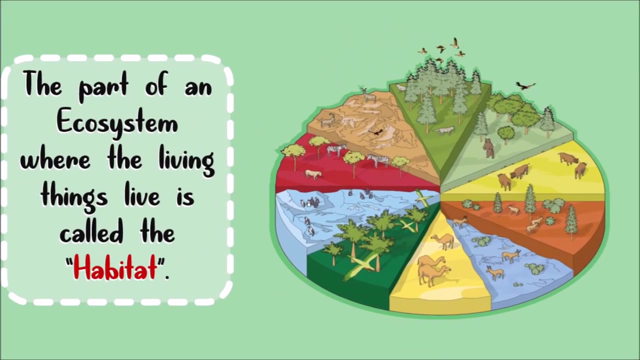 ecosystem's population and different population make up a community. the different populations in an ecosystem interact with each other and their environment. the living part of an ecosystem consists environment can be compared to marine animals, an arician or large ocean seal or bird living environment. in подум west, the part of the ecosystem where the living things leave is called the habitat. 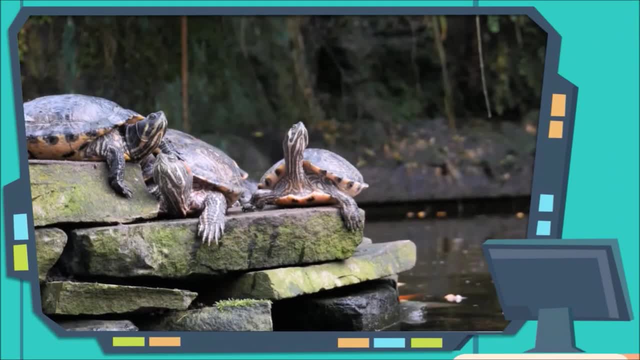 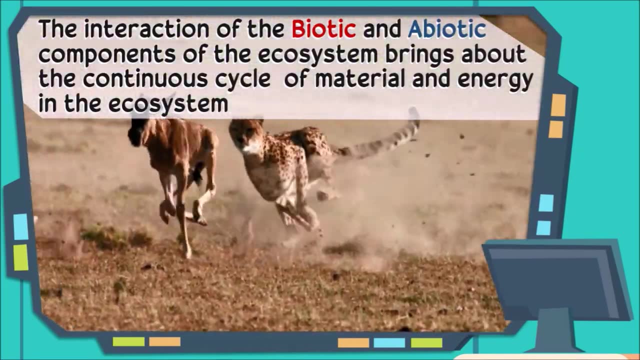 the radiation of Natasha's pristine water live itself in the composition ofkahwi. the interaction of the biotic and abiotic components, local ecosystems of the ecosystem brings about the Mother Earth comprehensive anabiotic dynamic cycle of materials of the ecosystem. brings about the continuous cycle of natural media, of romantic villages and of the ecosystem brings about the continuous cycle of materials, of natives and animals, 토, about mantenance of wildlife, about material and biodiversity- that is, a series of cycles. and of the ecosystem. brings about the continuous cycle of natural disasters that cause large size, Josh. and about the ecosystem, brings about the continuous cycle of natural disasters. that is, a series of Bull hinckley's powers that return to a 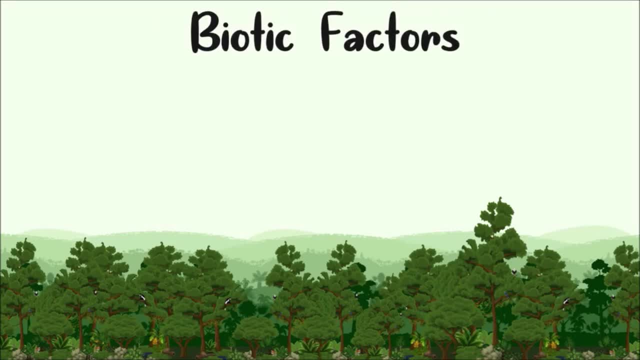 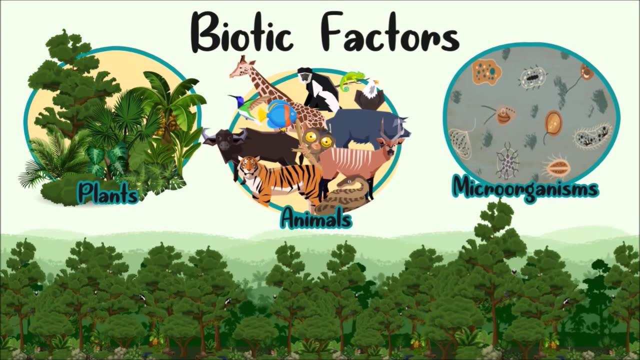 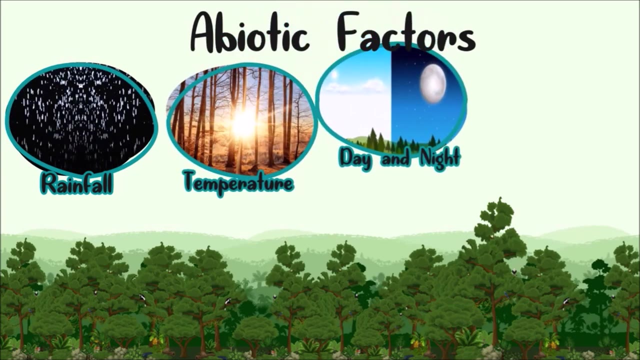 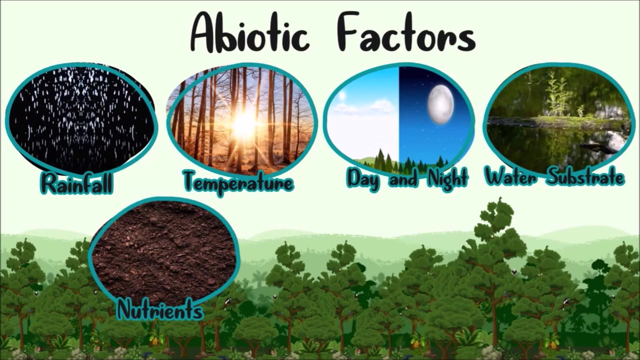 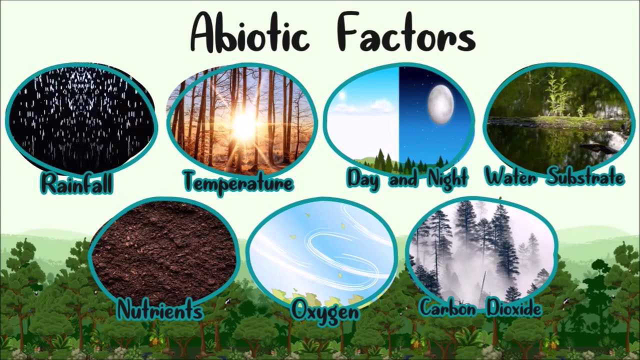 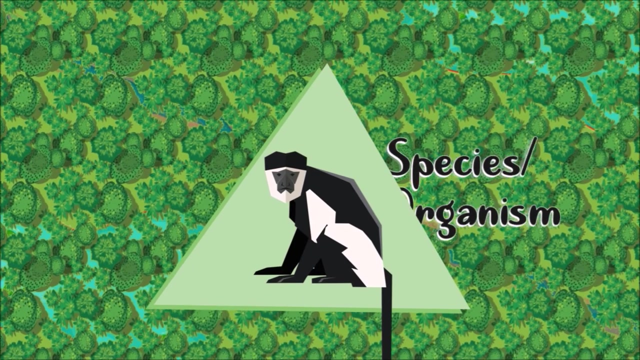 biotic factors may be plants, animals or other organisms. well, some examples of abiotic factors are rainfall, temperature, length of the day and night, water, substrate, nutrients, oxygen, carbon dioxide and many more. the living part of an ecosystem consists of different species or organisms. each species is a part of the 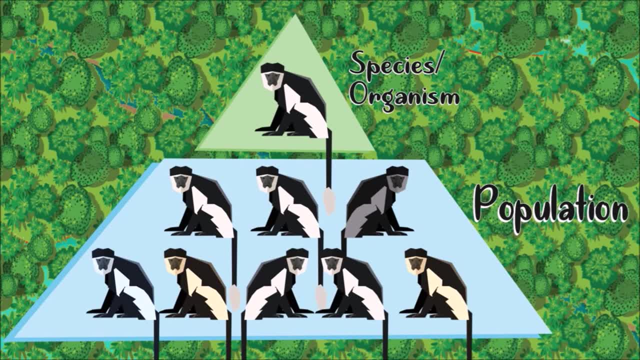 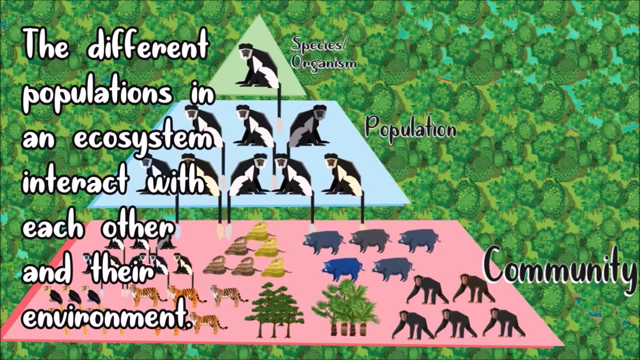 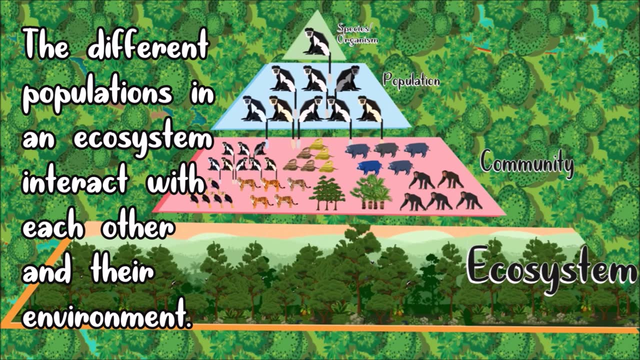 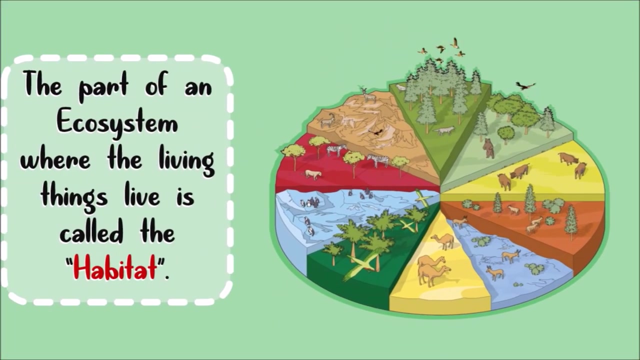 ecosystem's population and different population make up a community. the different populations in an ecosystem interact with each other and their environment. the living part of an ecosystem consists of different species or organisms. each species is a part of the ecosystem. the part of the ecosystem where the living things live is called the 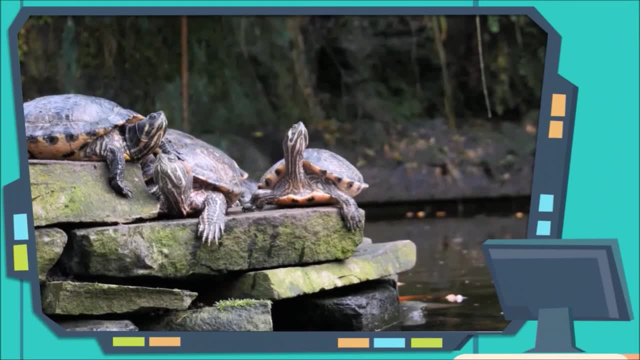 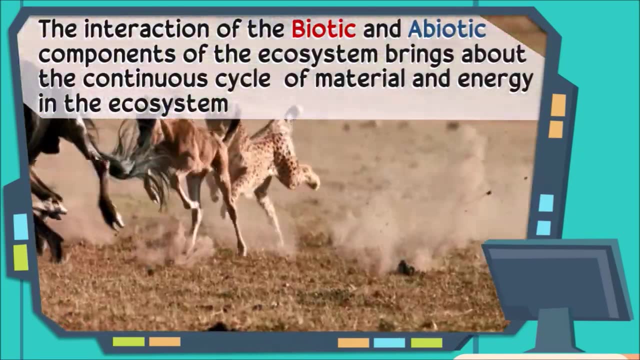 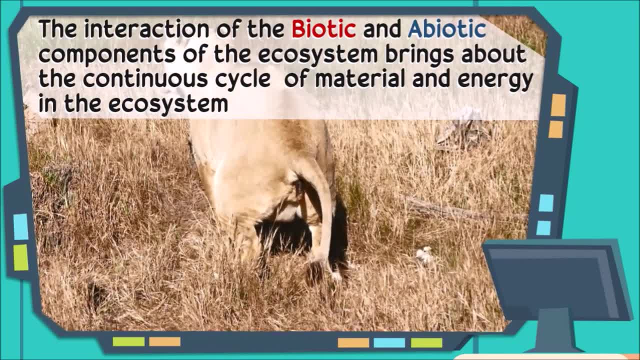 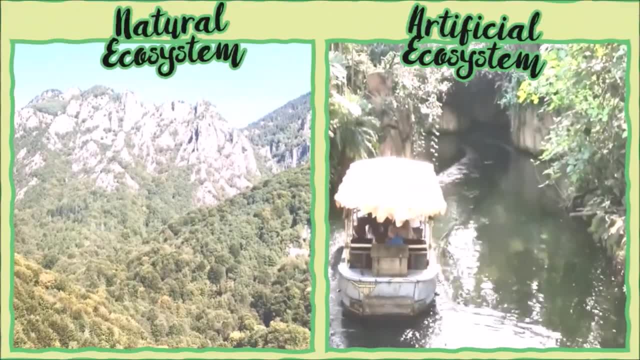 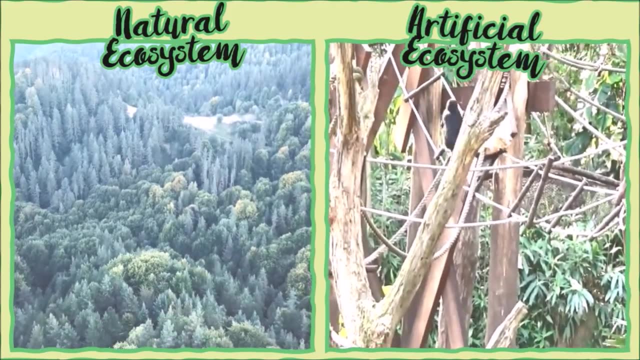 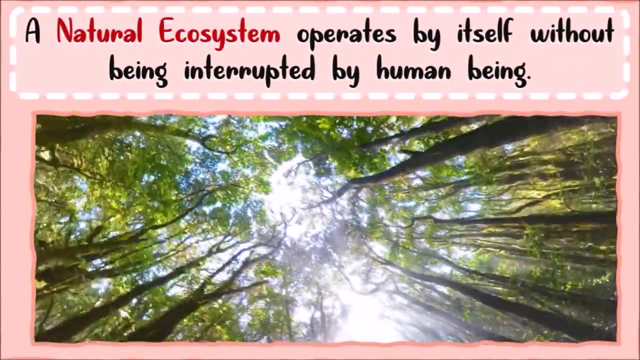 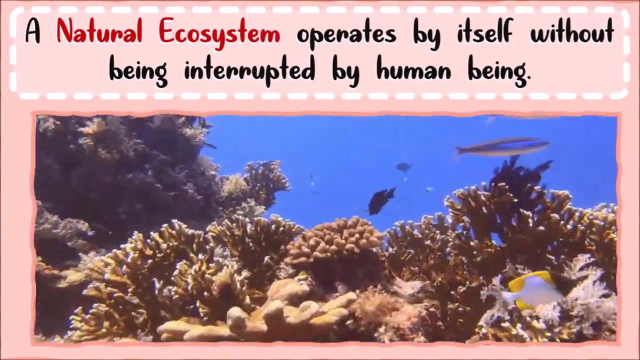 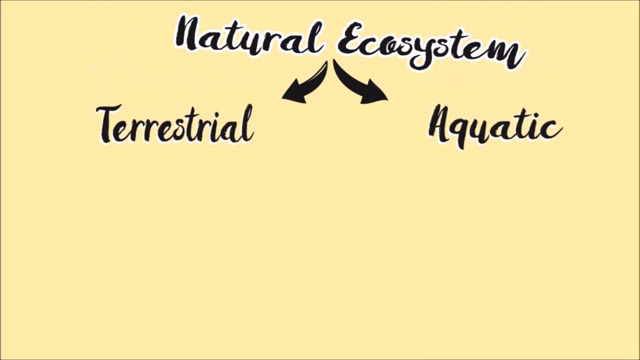 the interaction of the biotic and abiotic components of the ecosystem brings about the continuous cycle of materials and energy. energy in the ecosystem. an ecosystem can be natural or artificial. a natural ecosystem operates by itself, without being interrupted by human being. these type of ecosystem can be as terrestrial or aquatic. example of terrestrial 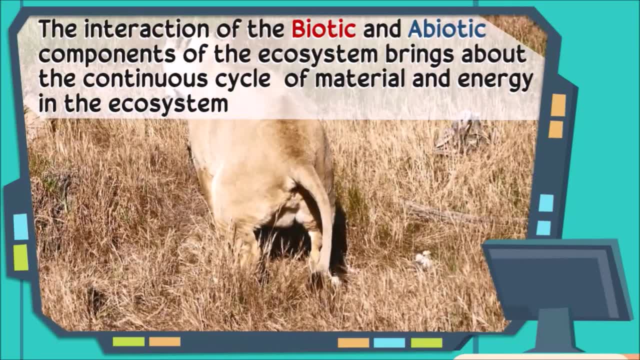 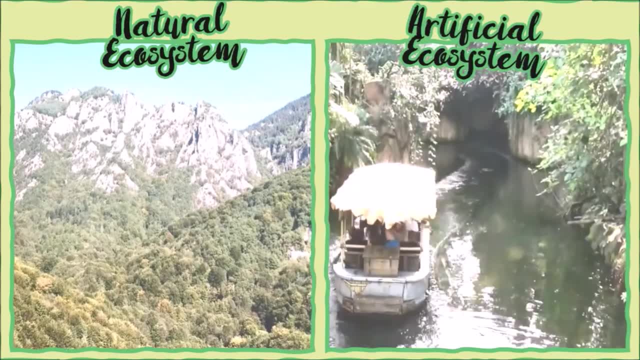 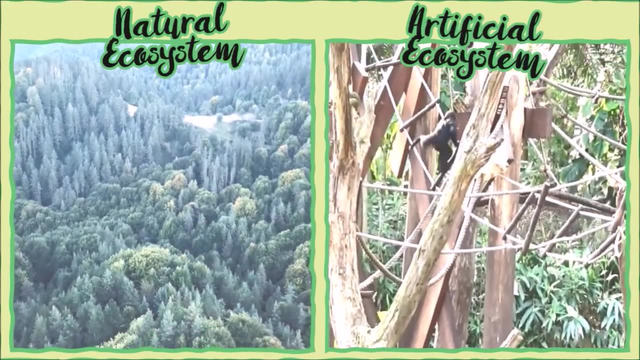 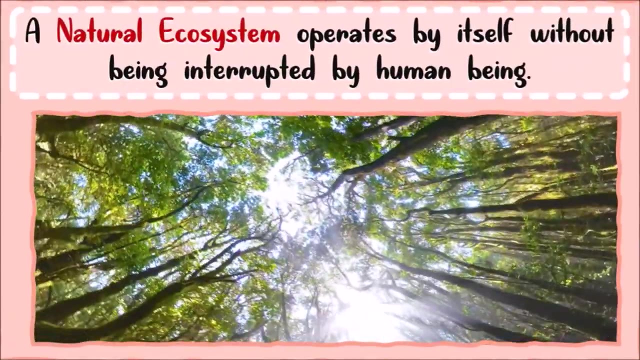 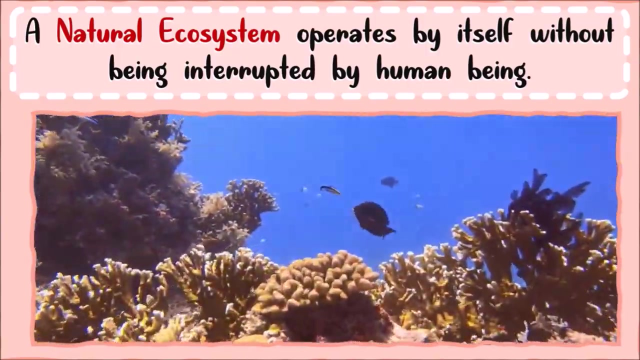 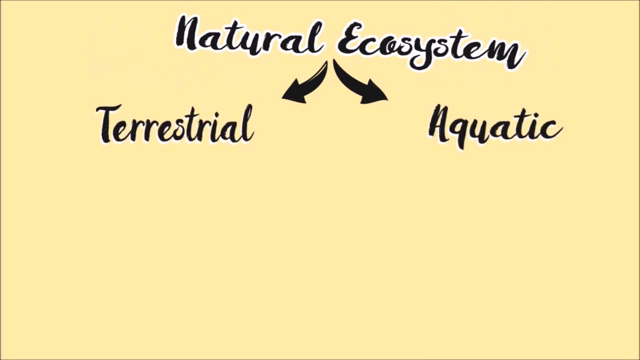 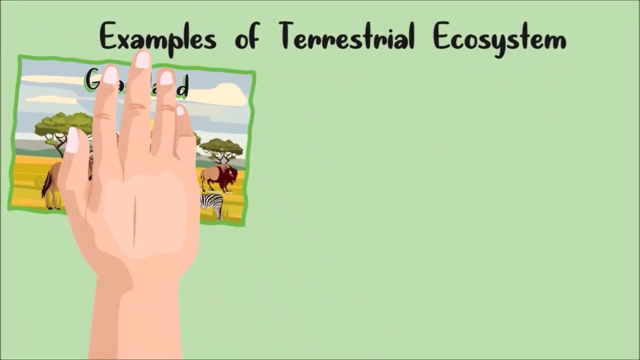 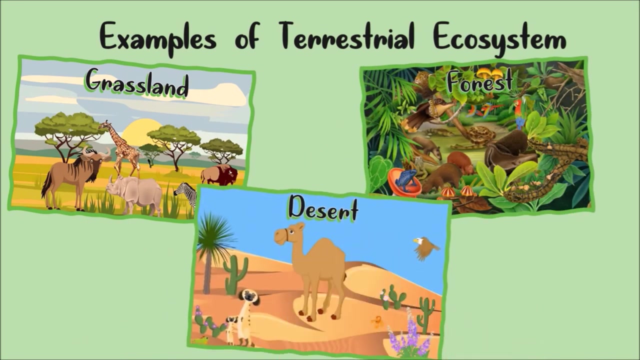 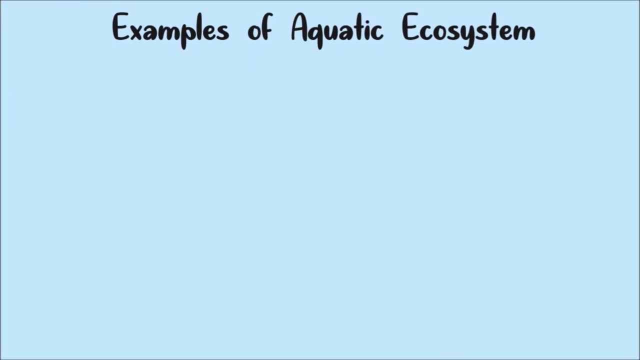 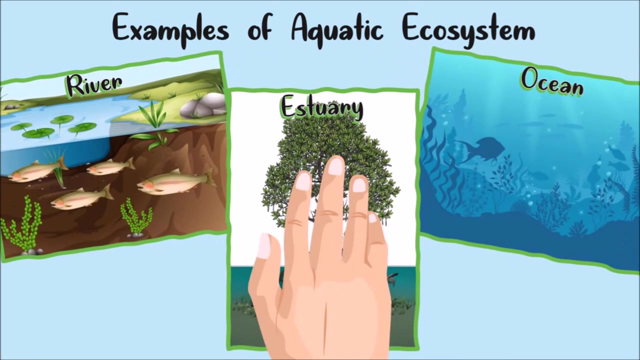 in the ecosystem. an ecosystem can be natural or artificial. a natural ecosystem operates by itself, without being interrupted by human being. this type of ecosystem can be as terrestrial or aquatic. example of terrestrial ecosystems are grassland, forest and desert, while examples of aquatic ecosystem are river, oceans and estuary. on the other, 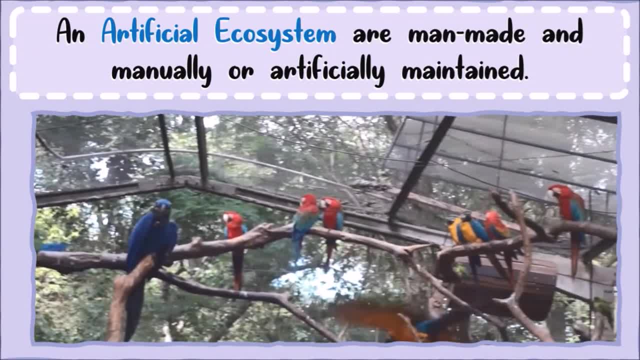 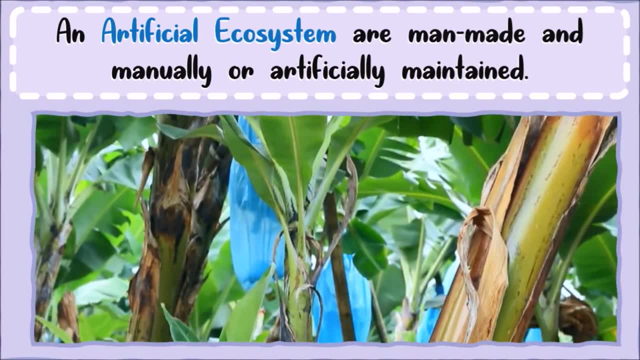 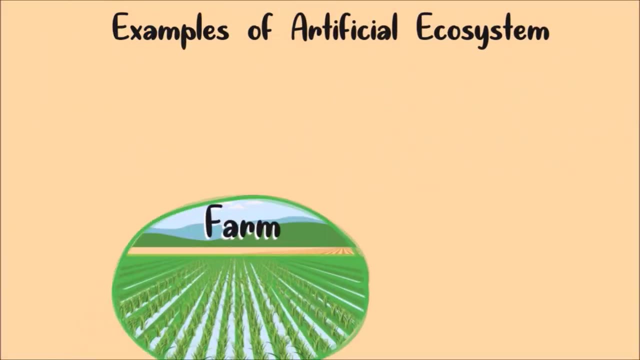 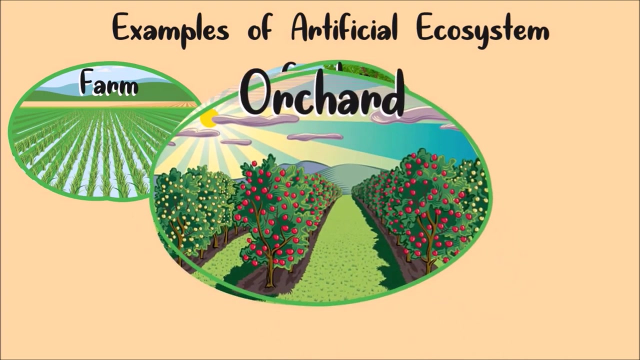 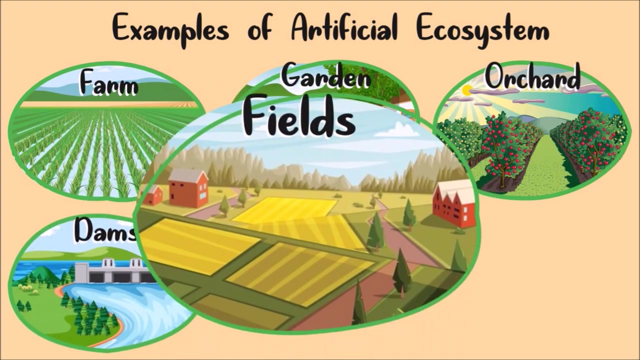 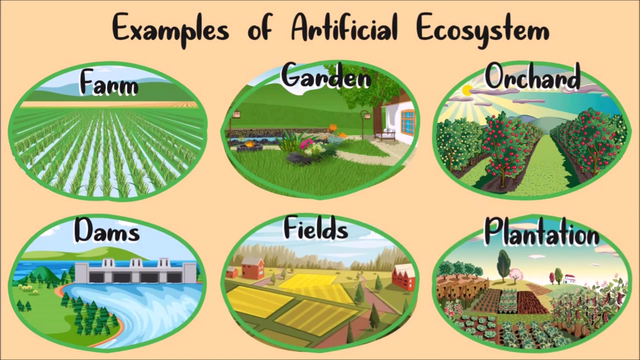 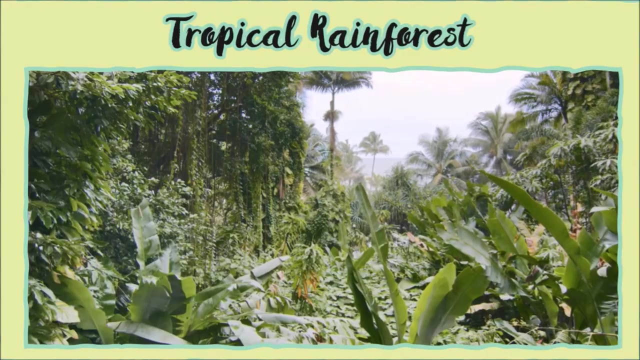 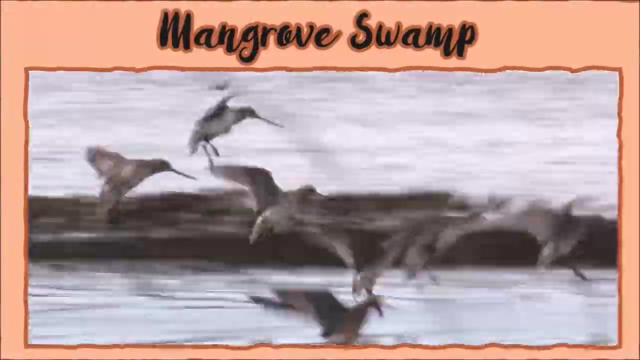 hand. artificial ecosystem are man-made and manually or artificially maintained. examples of artificial ecosystem are farm gardens, orchards, dams, fields and plantations. check out the next video about different ecosystem present in the philippines, such as tropical rainforest, coral reefs and mangrove swamp, and see the. 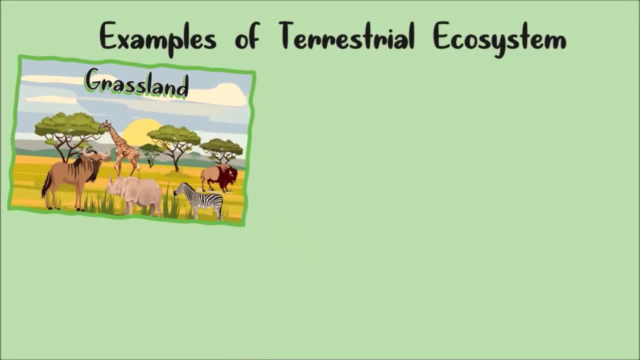 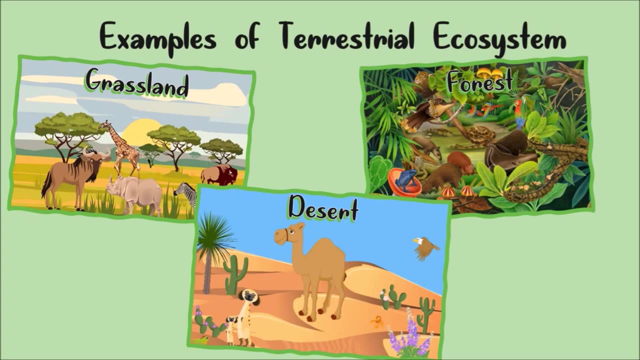 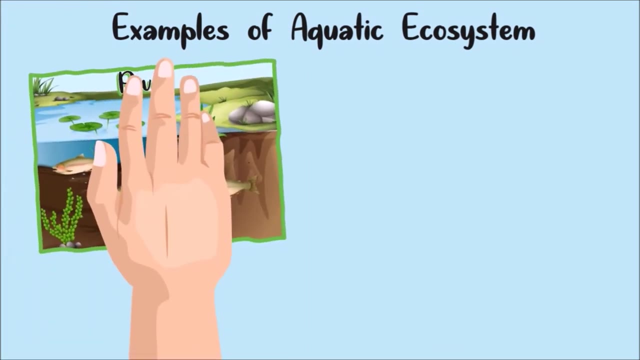 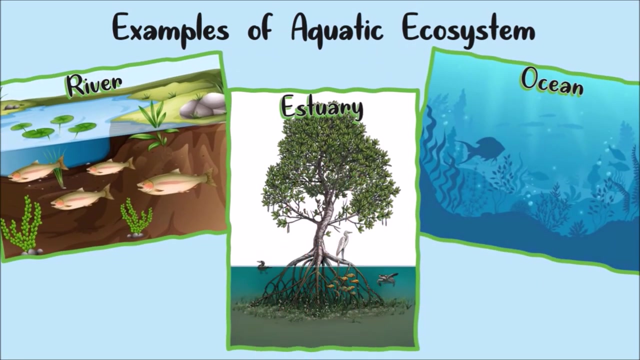 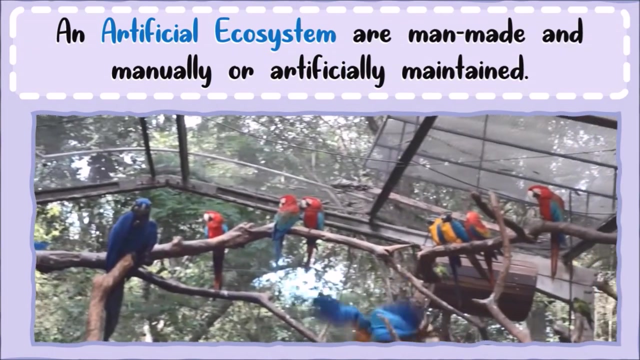 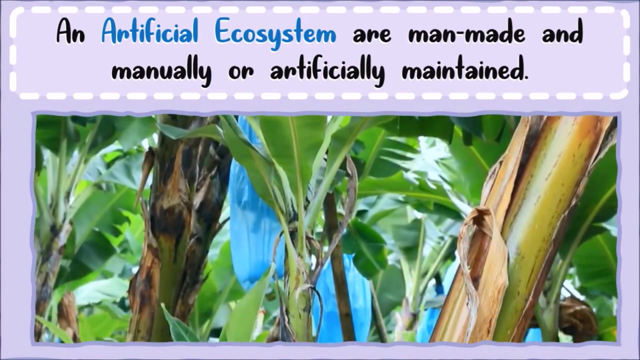 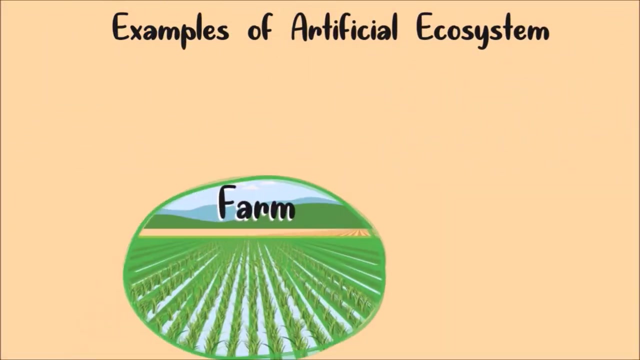 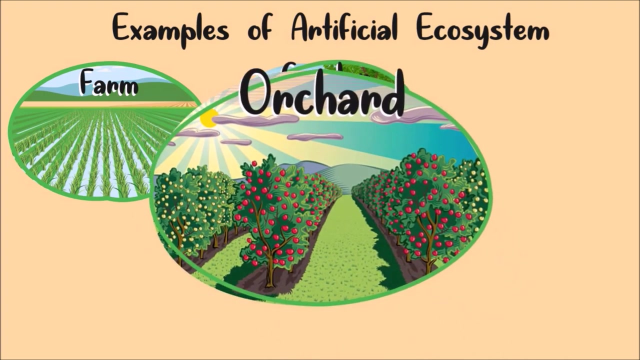 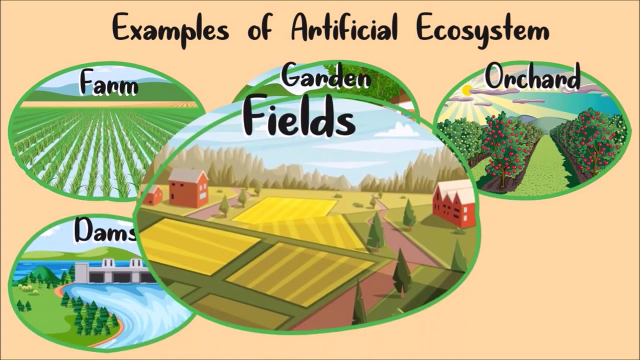 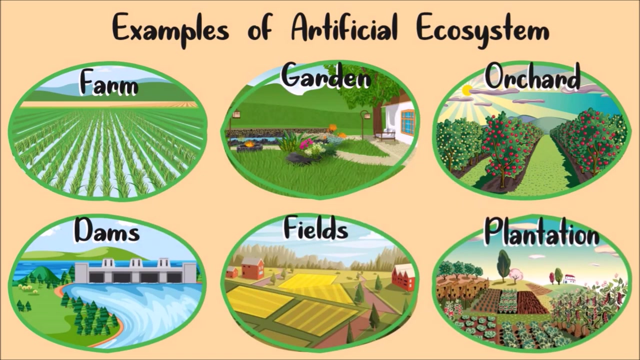 ecosystems are grassland, forest and desert, while examples of aquatic ecosystem are river, oceans and estuary. on the other hand, artificial ecosystem are man-made and manually or artificially maintained. examples of artificial ecosystem are farm gardens, orchards, dams, fields and plantations. check out the next video. 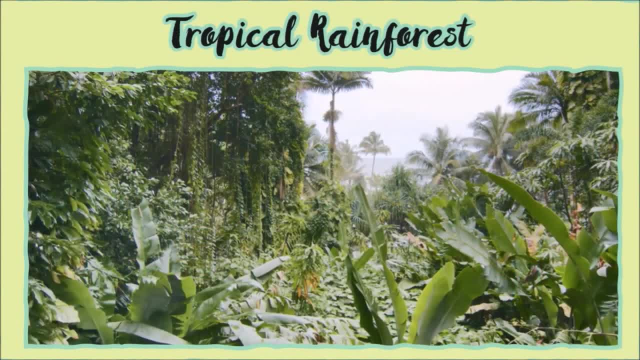 and plantations. check out the next video and plantations. check out the next video about different ecosystem present in the. about different ecosystem present in the. about different ecosystem present in the philippines, such as tropical rainforest philippines. such as tropical rainforest philippines. such as tropical rainforest, coral reefs.